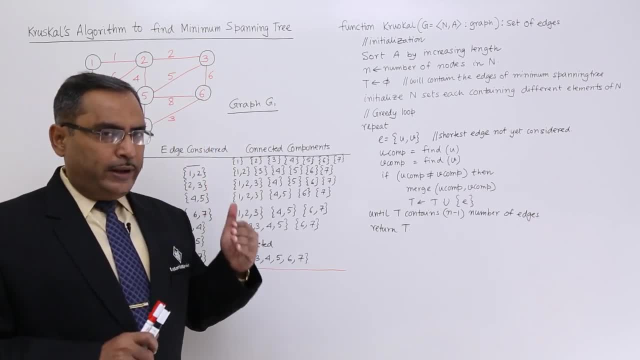 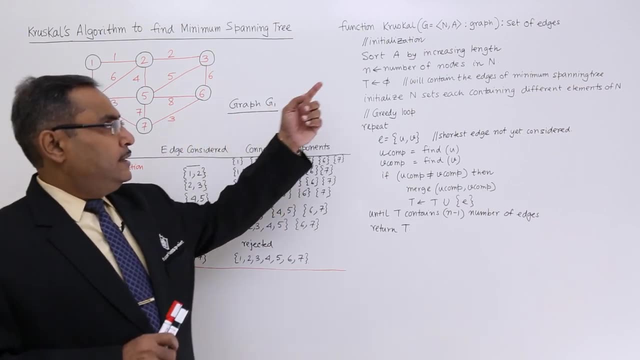 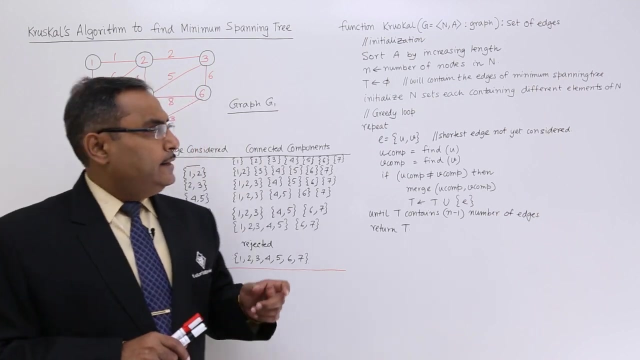 A by increasing length, So from the lowest length to the highest length. Length means actually weightage here. So we shall have to short all these edges. So A stands for edge, set of edges or arcs. N is the number of nodes in N. Here the value of N is equal to 7. T is equal to 5. So T. 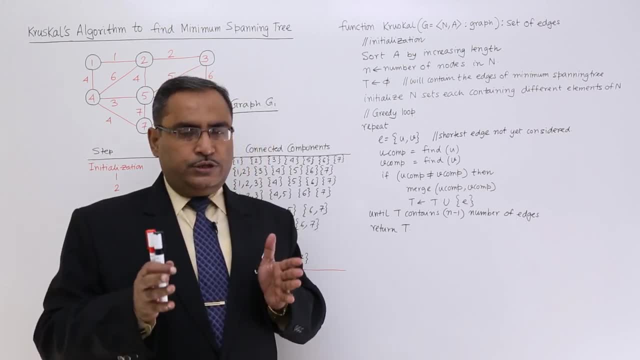 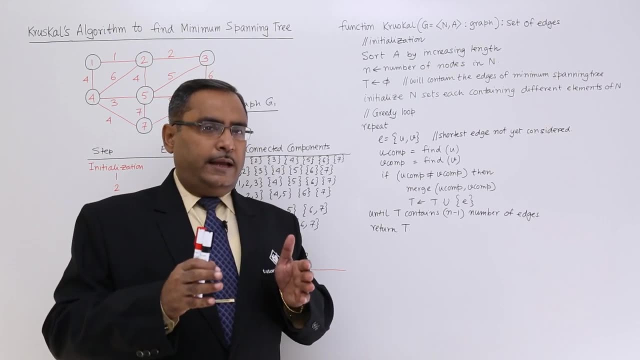 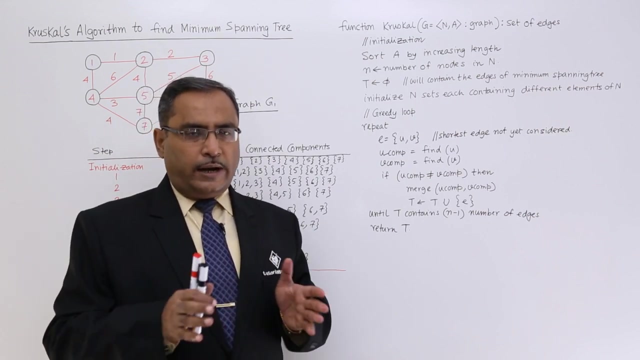 will be the result: holding set, which is containing all the sets which will form the minimum spanning tree Here we are having. N is equal to 7. So number of nodes is equal to 7.. So obviously we will be requiring 6 edges to connect them to form the minimum spanning tree. So the 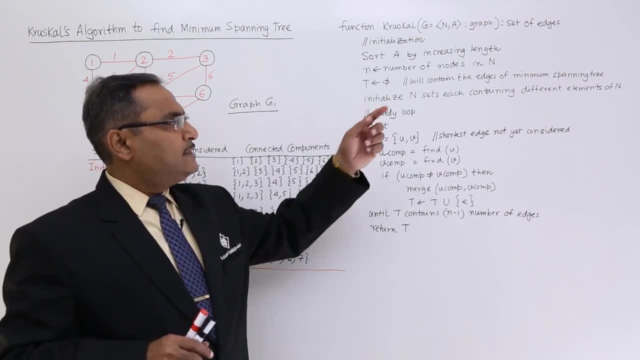 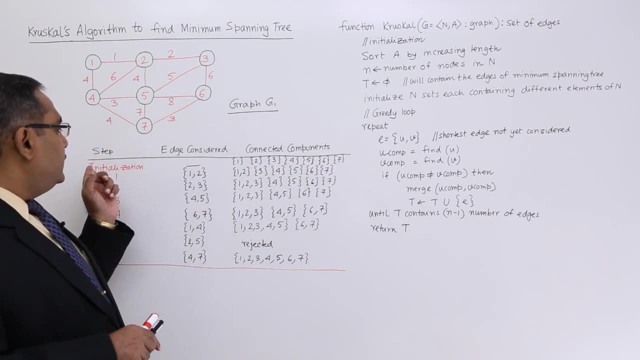 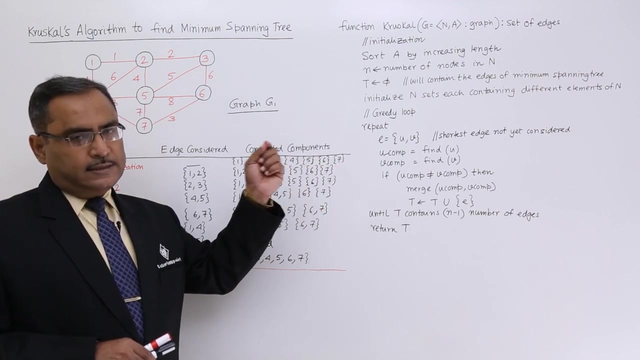 greedy loop is there. Next one is: initialize N sets each containing different elements of N. I have done this one here. I have done this one, So it is under initialization. I have done this one, So for each and every set we are having a distinct element of capital, N. That is the. 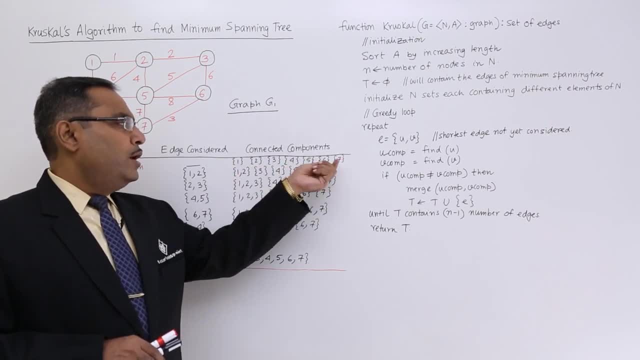 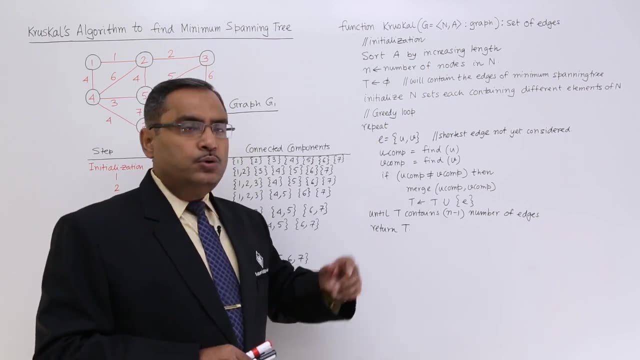 set of nodes. So set with node 1, set with node 2 and at the last, set with node 7, greedy loop: repeat. So now E is equal to UV, E is equal to UV. So this is the initialization. 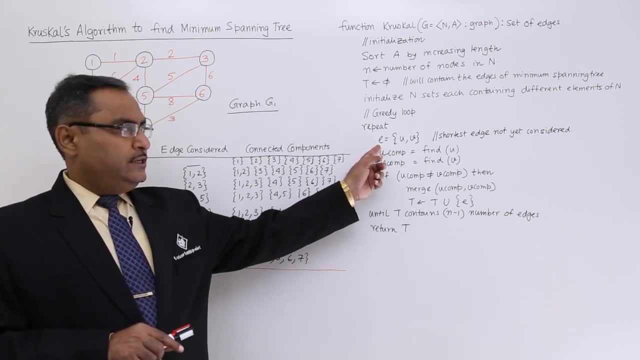 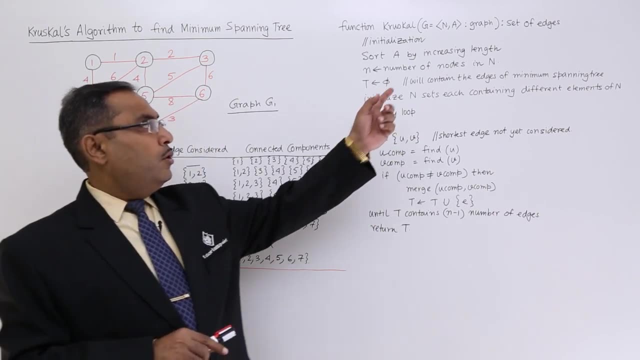 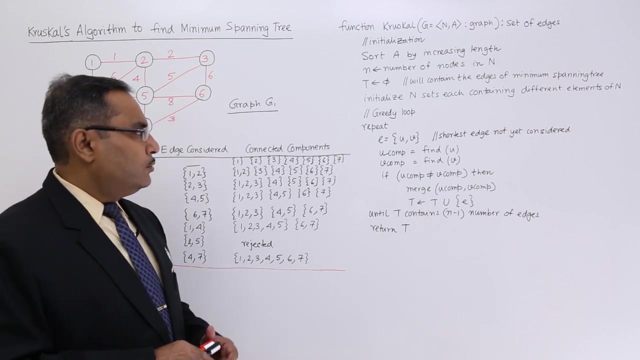 So e is that very edge which is connecting nodes u and v. shortest edge not yet considered because already we have done the shorting in the ascending order. So shortest edge not yet considered. now see, here we are having considering full graph, we considering that. 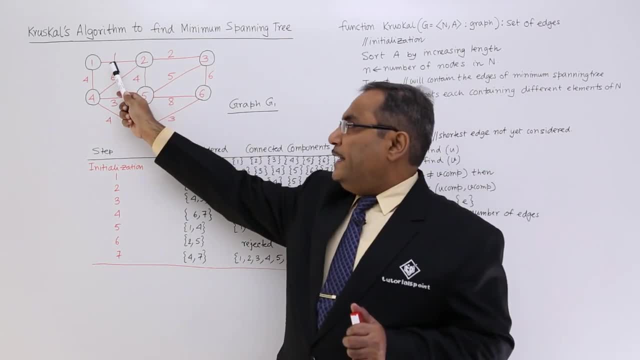 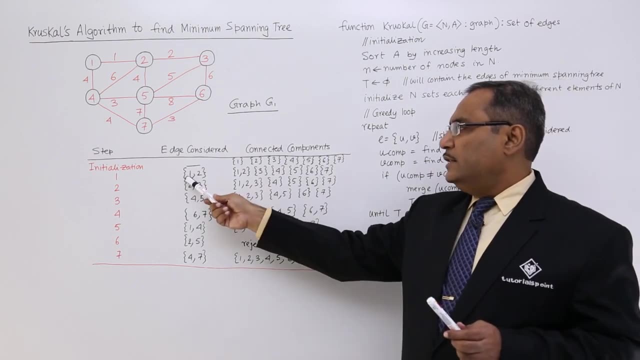 u is equal to 1 and v is equal to 2, with the edge weightage with 1.. So that is the shortest one, or the minimum weightage. we are finding this one. So we are considering this one, 1 and 2, this edge, we are considering. you see, 1 is a member of this set and 2 is a member. 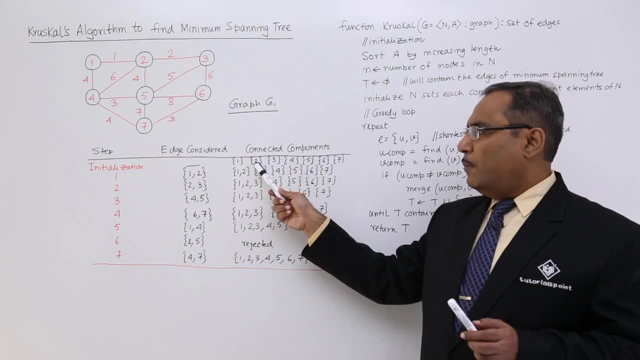 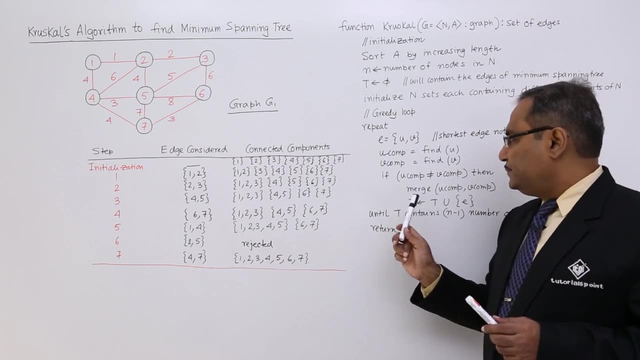 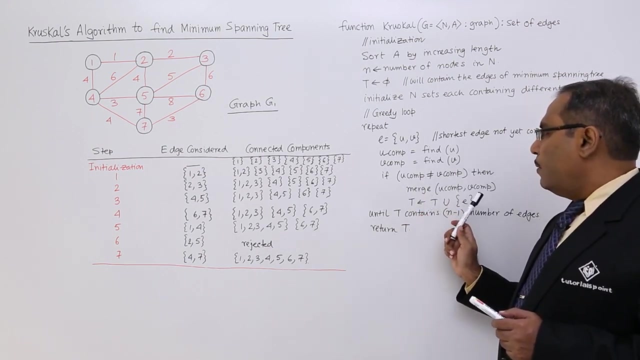 of this set. So that is the u comp and this is the v comp. So they are not equal to each other because they are from the different sets. then what they are doing they are just when these two, u comp and v comp. when they are not equal, then merge u comp, v comp. So 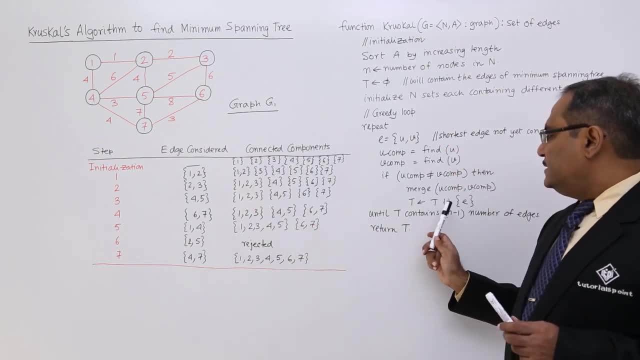 this: 1 and 2. this two set has to be equal to 1 and 2.. So this set has to be equal to 1 and 2. this set has got merged and t is equal to t, union e. So t is the output, that is. 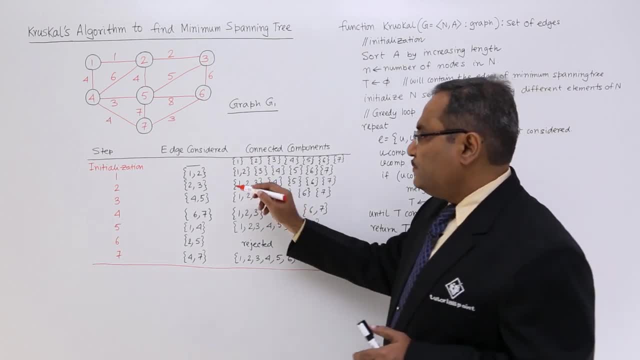 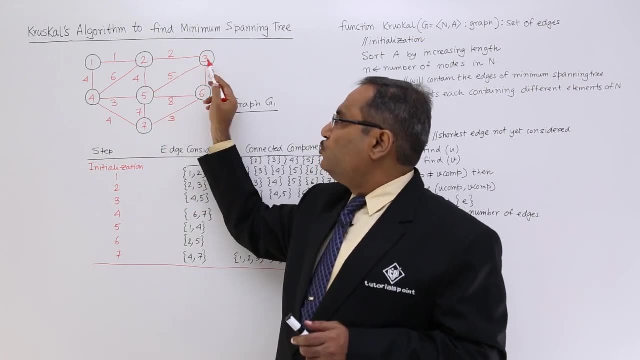 the set of edges, that is the minimum spanning tree edges. So this particular edge has been considered next. So, considering them, anyone, we are having this one, So 2, 3.. So 2 is belonging to this particular set and 3 is belonging to this particular set. say u comp. 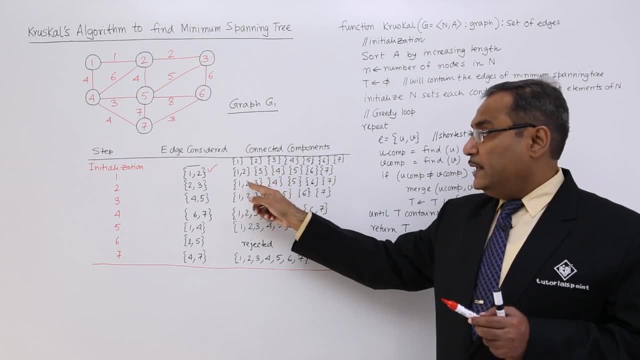 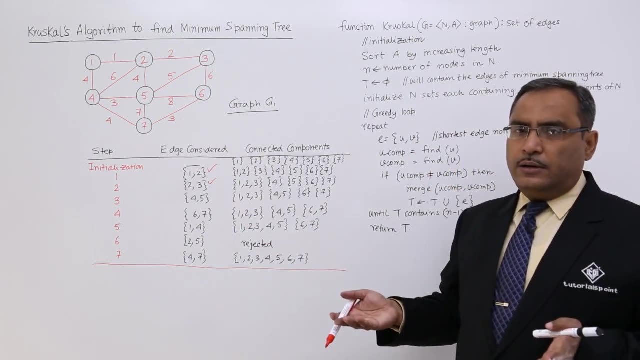 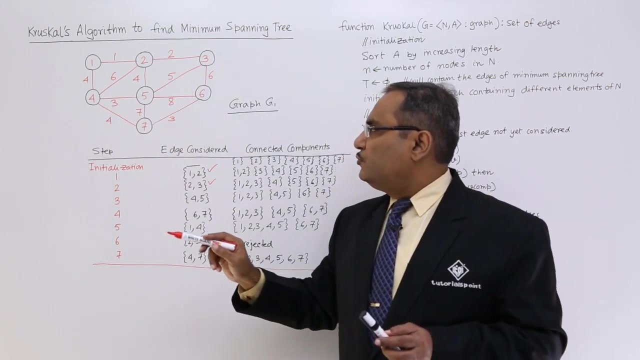 and v comp. they are not equal, So that is why they- these two sets, will be merged and this particular set, So this particular edge, 2, 3 will be considered Similarly. we are going for the rest. So any anything. yes, we are having this 4- 5. we are having this 4: 5 with the weightage of 3.. We 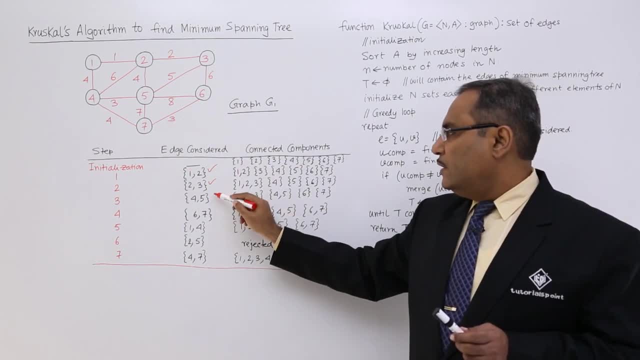 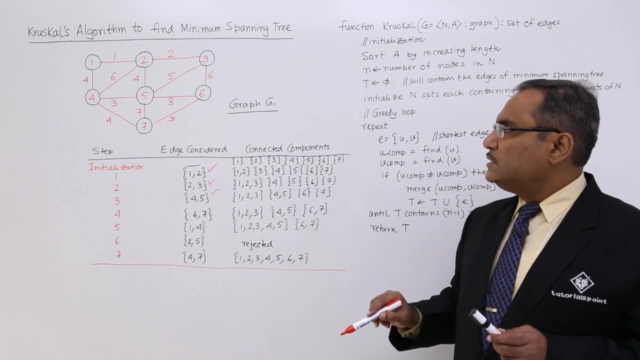 could have considered this: 7, 6 also, So 4, 5.. So 4 is belonging to this set, 5 is belonging to this set, So they have got merged. So now 4, 5 has been considered. Now see any edge. 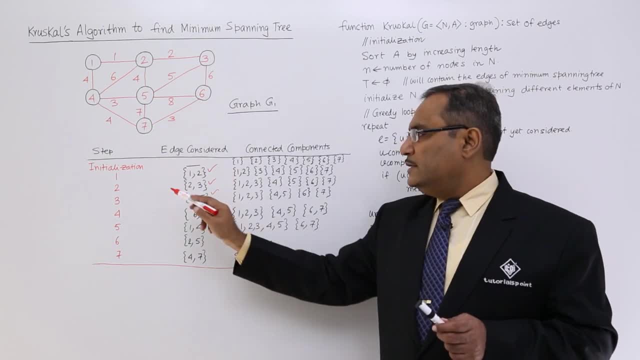 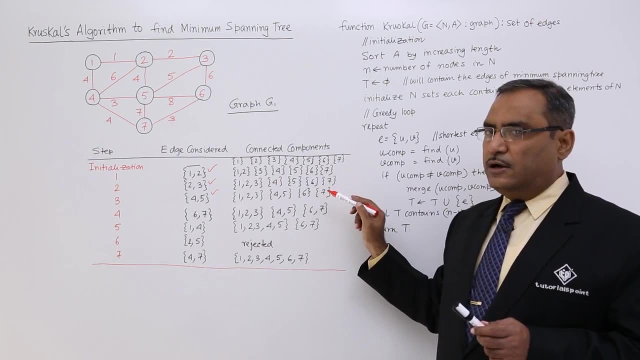 with the minimum weightage 6- 7.. So now we are considering 6- 7.. So 6- 7 is belonging to this set, 7 is belonging to this set. They are this: these two sets are not same, So they are going to be get merged and we are considering this one and 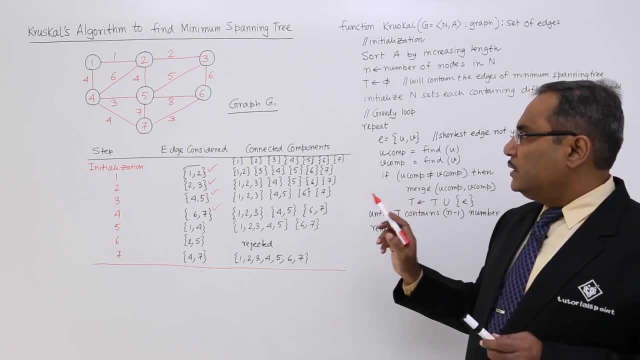 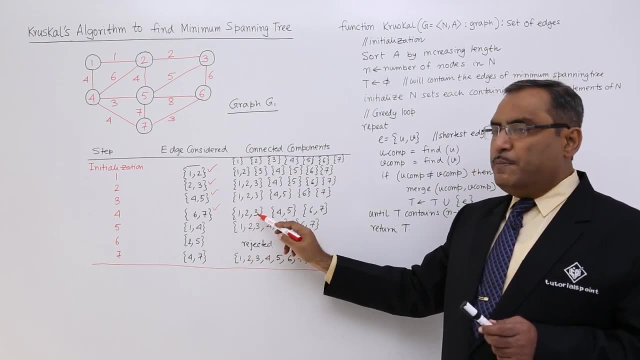 putting it in e, after doing the union operation. So 3. so there is a weightage 3.. Now we are going for 4.. So 1- 4. I am taking this 1, 4.. 1 is the member of this set and 4 is. 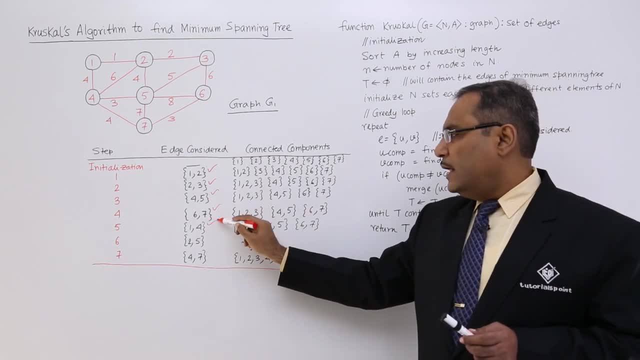 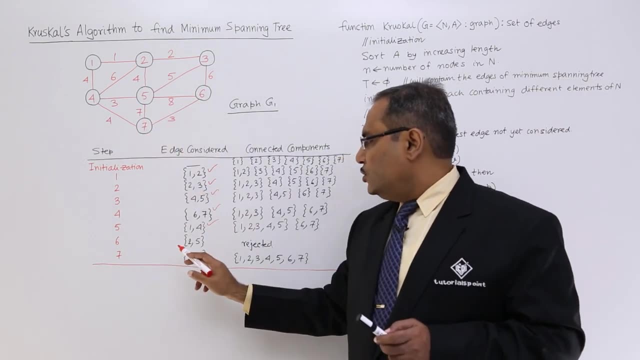 the member of this set, So please merge them, and this is my considered edge. This is the. So now any 4. yes, we are having this- 2, 5.. So 2 5, 2 is belonging to this set and 5 is. 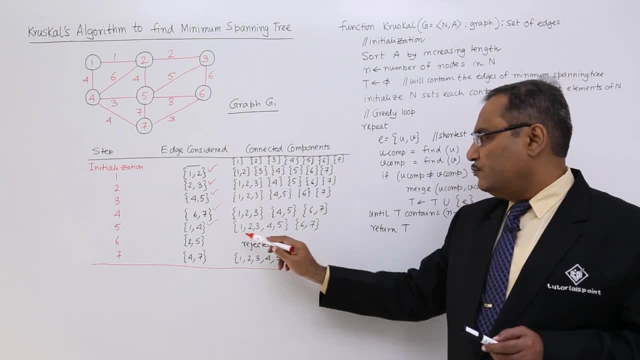 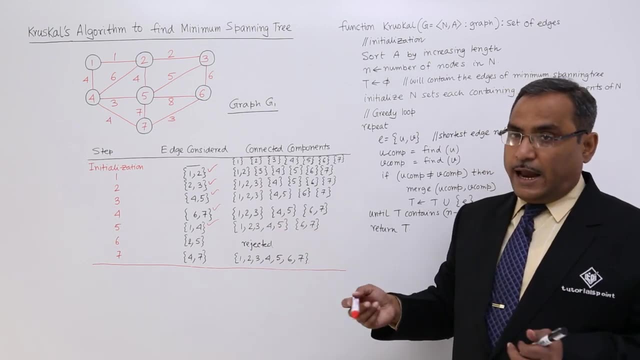 also belonging to this set. So sorry, 2 5, 2, 5 is this one. So now you see 2 and 5. both are belonging to the same set, So that means they cannot be merged. So if they are not, 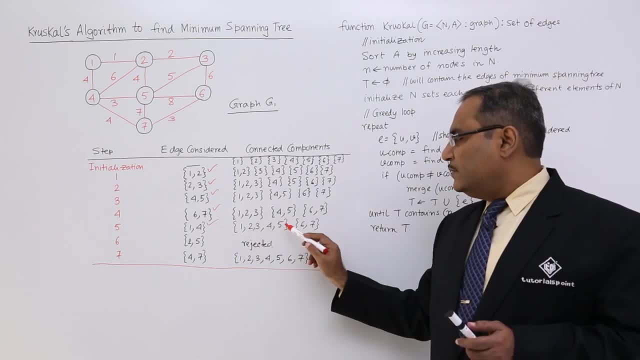 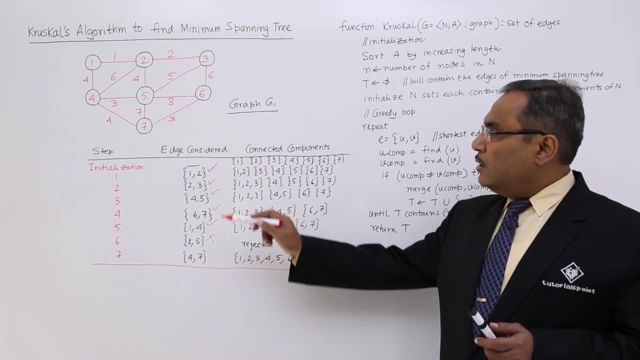 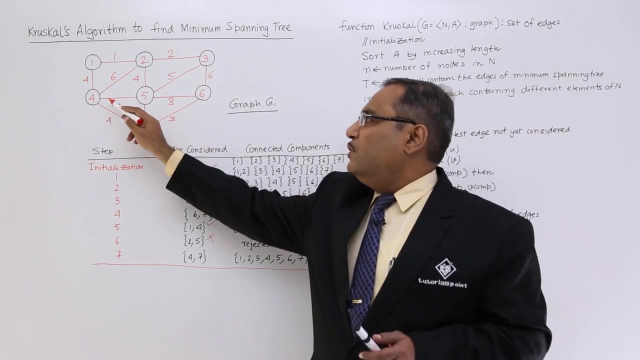 equal, then you are doing so. but as they are from the same sets- 2 and 5 both- So this particular age is getting rejected. So now, 2 and 5 means what is the weightage? what was the weightage is? weightage is 4.. Next one is my 4- 7.. So that is having also weightage. 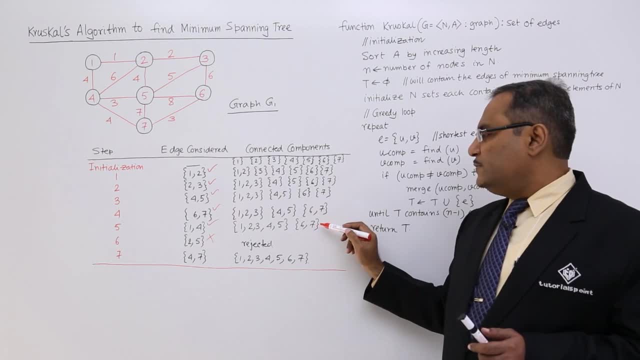 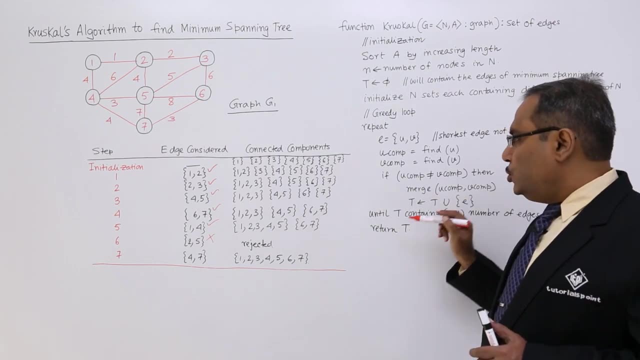 4.. So 4, 7: 4 is belonging to the set and 7 is belonging to the set, So they, these 2 sets, are different, So please merge them as they have told. So now they have got merged. 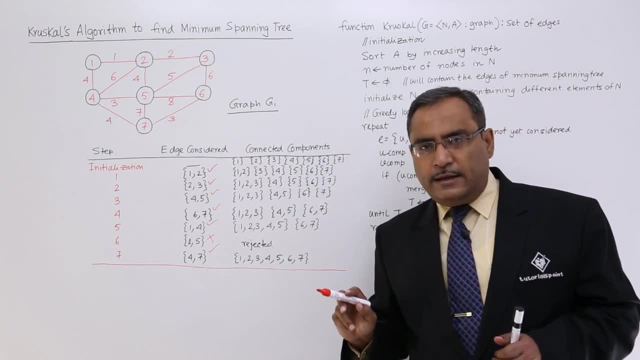 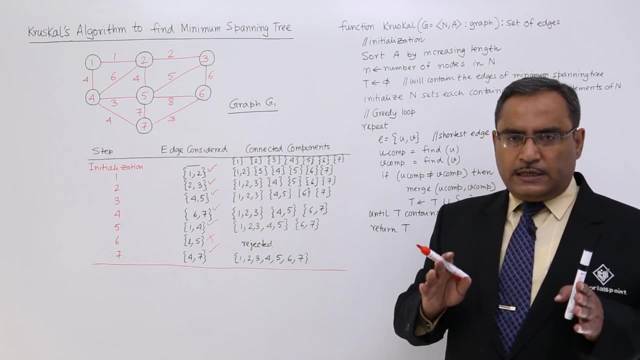 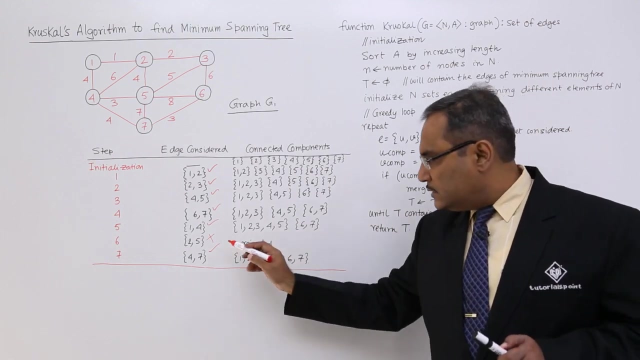 and I am considering this one. So now here the value of n, that is a number of elements in capital N. So capital N is 7, because we are having 7 nodes. So to form the minimum spanning tree we require 6 edges: 1, 2, 3, 4, 5. we have already considered 6.. So already considered 6 edges. 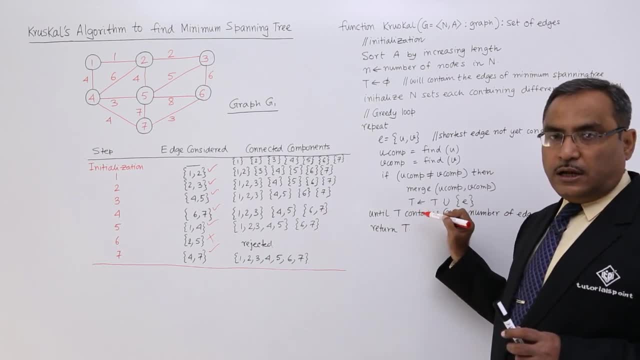 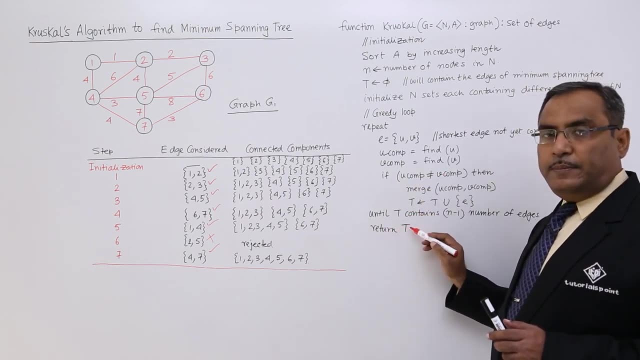 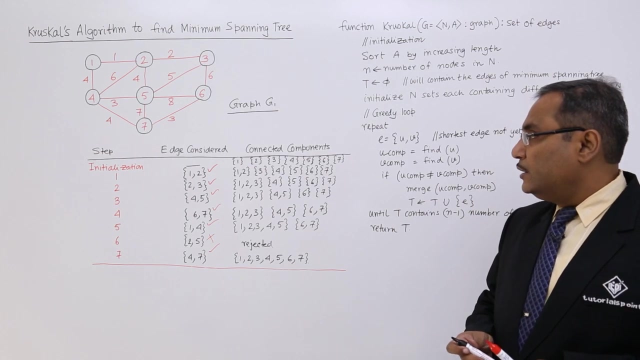 So that is why. So this particular condition is now allowing it to come out from this repeat until and return t will take place. So in this way, the things will take place. So now, let me mark that. So let me mark that, what edges we have considered ultimately? So, edge in between 1 and 2, 2, 3.